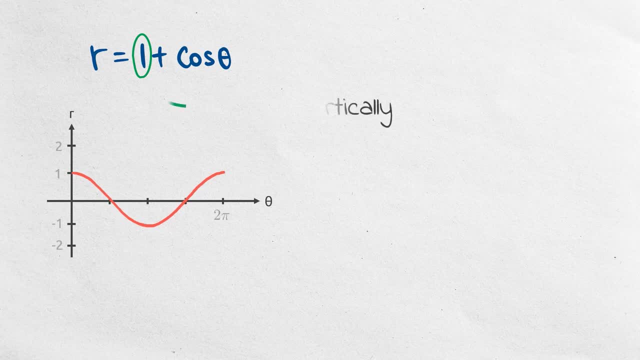 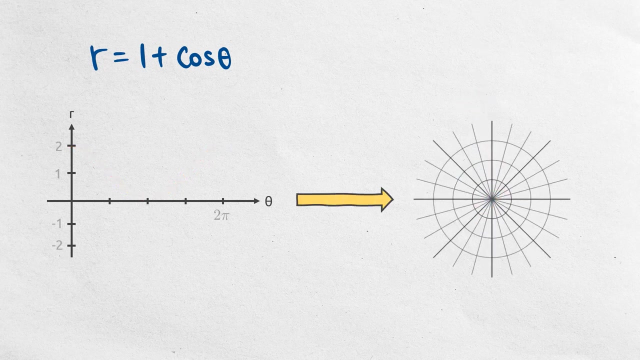 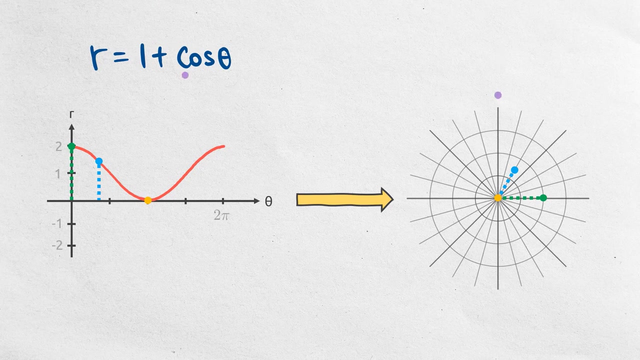 The 1 in the equation shifts the basic cosine graph one unit up vertically. So that's our polar equation plotted in the rectangular plane. Now how does this graph help us graph the cardioid more easily? Here's the idea. The vertical distance between each point on the graph and the x-axis is how far each polar point. 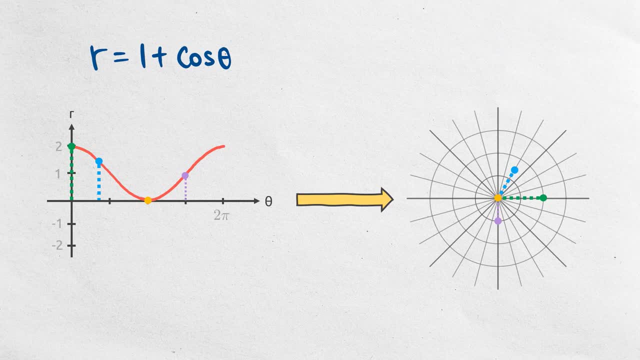 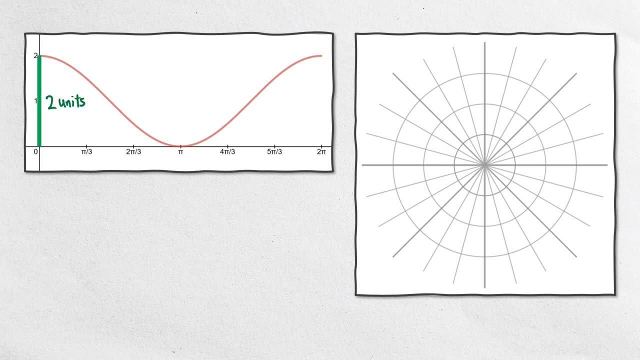 is from the origin. Using this idea, we can start graphing. Starting with theta equals 0, we see that the vertical distance is 2.. So r is 2 and theta is 0. Plot the point with a distance of 2 units from the origin when theta is 0.. Other points that are extremely easy to plot: 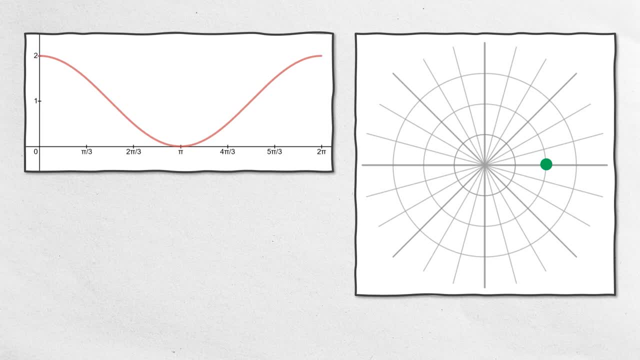 are pi over 2,, pi, 3pi over 2, and 2pi. We see that at pi over 2,, r is 1.. At pi, r is 0.. At 3pi over 2,, we get r to be 1.. Coming back to 2pi, we get 2,, which is our starting point. 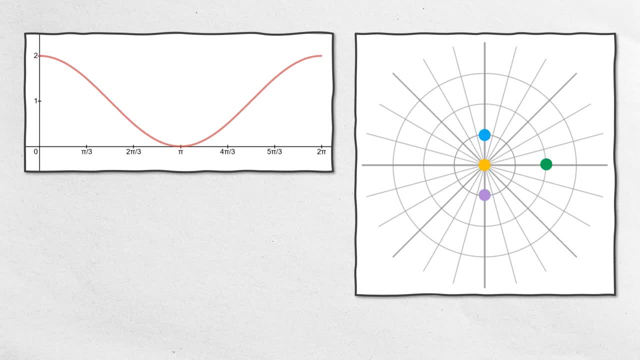 Now, only having these 4 key points may not be enough to graph the polar curve, So we start looking at some other points. For example, we have to graph the polar curve from the origin to the origin. For example, from the graph we can see that we have a y value of 1.5 at pi over 3.. So 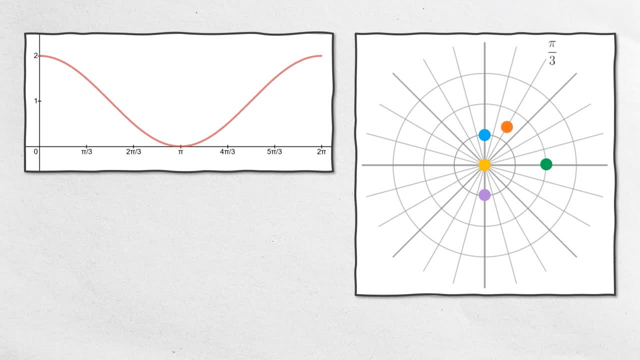 we have a point 1.5 pi over 3. And by symmetry we get another point here. In fact, we may not always get nice values like this, So we usually try to approximate. Here's how we can do that. 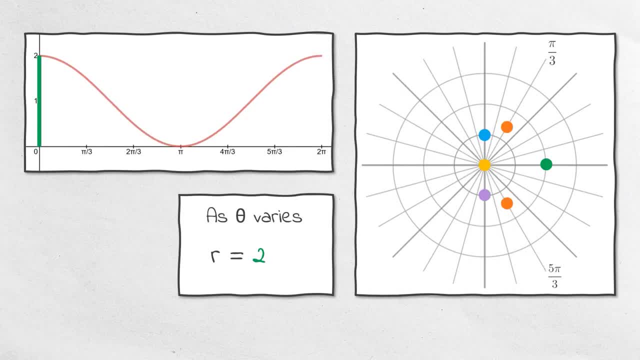 Starting from the initial point, we see that the y value starts at 2, and starts decreasing. So, on our polar plane, we start drawing the curve by going in the counterclockwise direction, and we need to make the distance from the origin smaller and smaller. 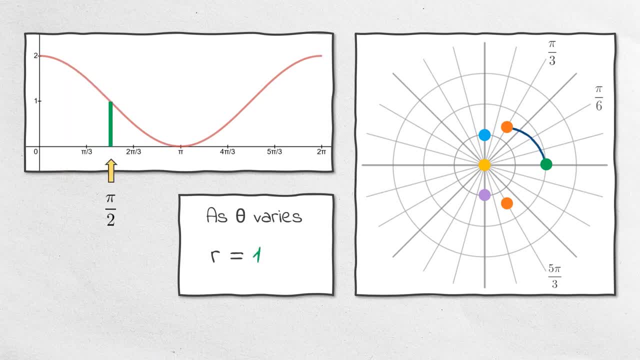 See that all the distances from the origin will be decreasing from 2 to 1, as we get to a key point: 1, pi over 2.. Getting past pi over 2, the y values are getting smaller from 1 and decrease to 0,.